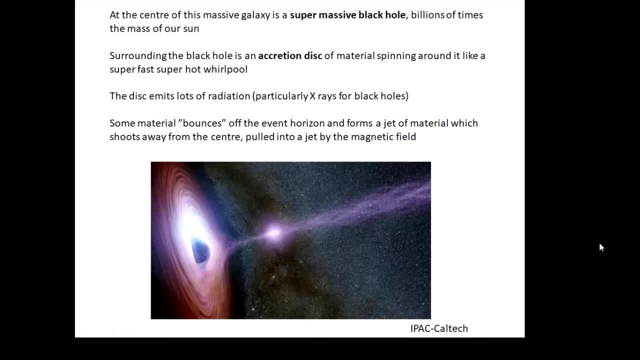 Some of them are ridiculously big, billions of times bigger than the mass of our sun- Huge black holes, And surrounding the black hole is an accretion disk, a disk of stuff whizzing around very, very fast. A superfast, hot whirlpool of stuff whizzing around. 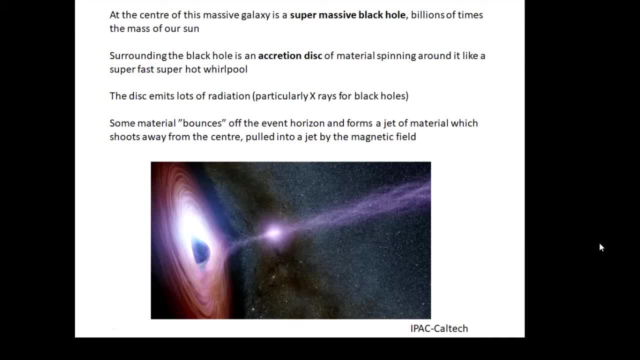 Okay, that's the accretion disk, And when stuff whizzes around like that it gives off lots of radiation, particularly x-rays for black holes. There's different types of accretion disk And basically the hotter it is, the more of the higher wavelengths it gives out. 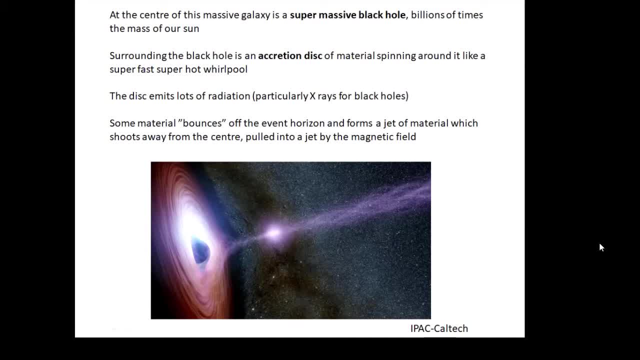 Something like the accretion disk around a protostar gives off lots of infrared, But around a black hole we're talking x-rays, X-rays and gamma rays as well. Now, some material doesn't get sucked into the black hole. 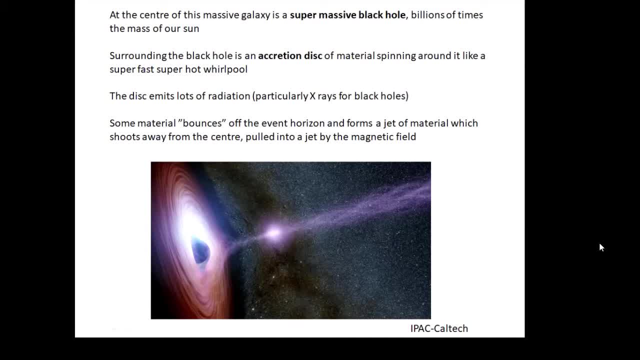 What happens is it bounces off the event horizon very, very fast And it forms a jet of material which shoots away from the center And the magnetic field of the black hole helps it to form. It collimates- it is the word- into a jet of material stretching out hundreds of light years from the black hole. 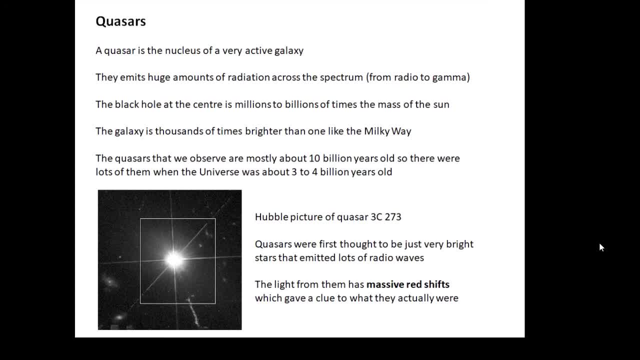 Quasars. What is a quasar Now? the quasar is the nucleus of a very active galaxy. They emit huge amounts of radiation across the spectrum. You know all the way from big wavelength radio to small wavelength gamma. Lots and lots of radiation. 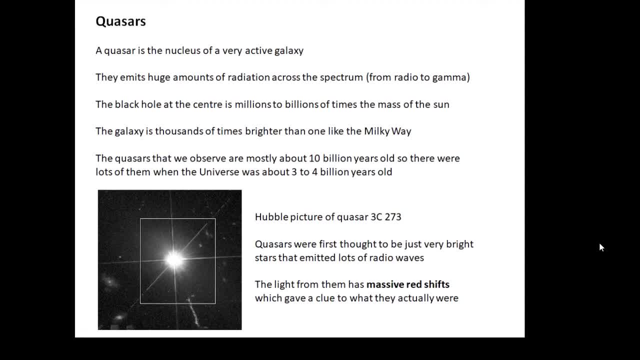 At the center is a black hole, millions to billions of times the mass of the sun. So we're talking about a black hole. We're talking a massive, massive nucleus, A very, very active, big nucleus. The galaxy is thousands of times brighter than one like the Milky Way. 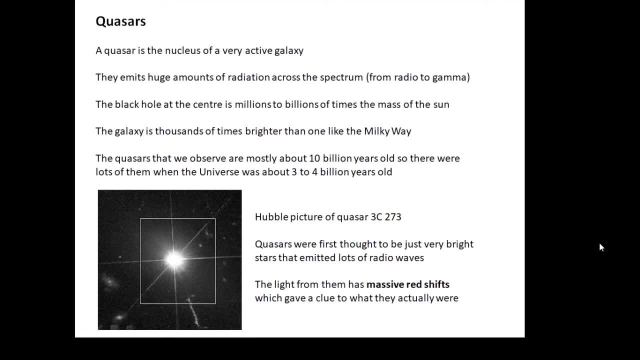 The quasars that we observe are mostly about 10 billion years old, Because they're about 10 billion light years away, And this means that when the universe was about 3 to 4 billion years old, that was the epoch of the quasars. 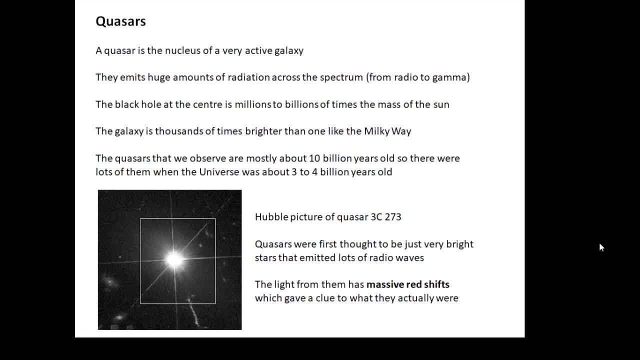 There were lots of quasars. There were lots of quasars around at that time. This is a Hubble picture of a quasar. Okay, It looks like a very bright star, But it's also giving off lots and lots of radio waves. 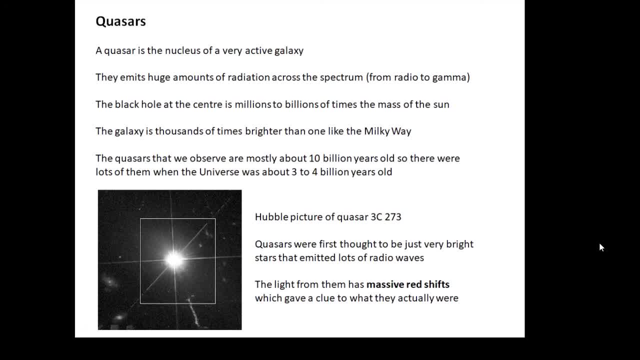 Sometimes astronomers just detected the radio waves And they were wondering where it was coming from. So it was a quasar, stellar object, A quasi-stellar object, A quasar. Is it a star? We're not sure. It's a quasi-star. 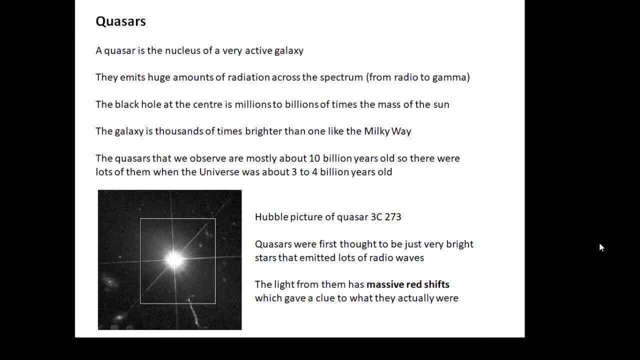 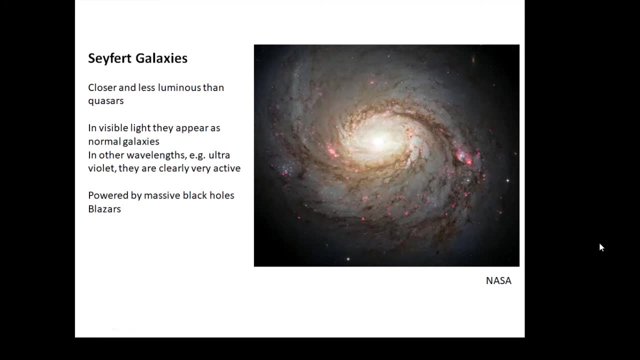 The light from these quasars has massive redshifts And we'll learn from topic 16 that this tells us they are very, very far away. Quasars, Seyfert, galaxies- they are quasars' little brother. 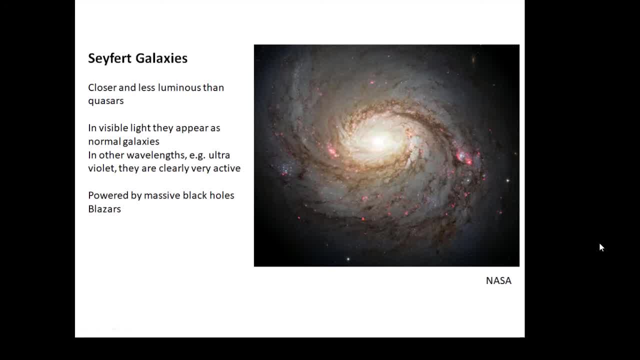 They are not as far away as quasars. They're not as luminous as quasars. They still give off lots and lots of radiation. They're still active galaxies. Okay, In visible light they look like normal galaxies, But if we look at them in other wavelengths we see that their nuclei are very, very active. 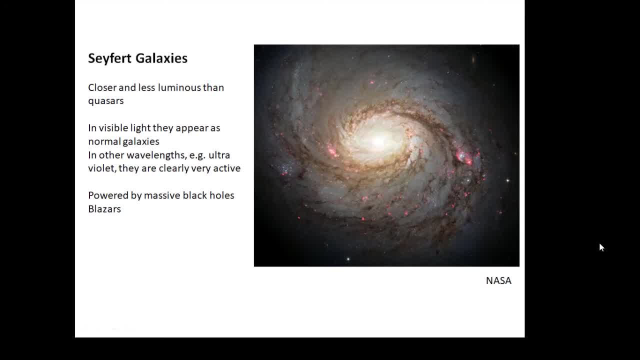 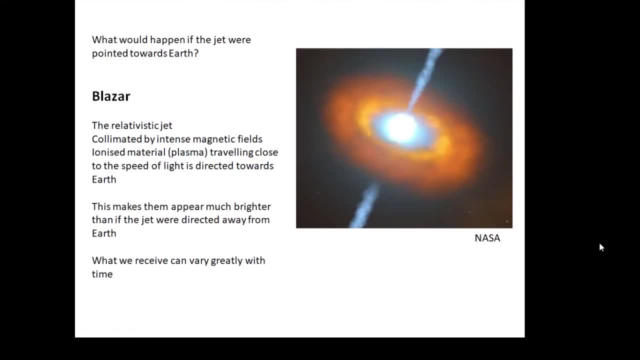 In the middle of them, there is a massive black hole. Okay, Which moves us on to blazars, which is the last slide. Now, what would happen? We talked about this jet And all of this radiation being given off. 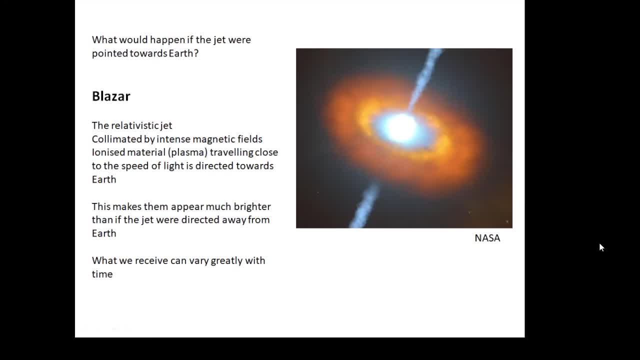 What would happen if it was pointed towards the Earth? Well, if it was pointed towards the Earth, that is a blazar, And the fact that the jet and all of this radiation is heading towards Earth makes them appear much, much brighter than if the jet were pointing away. 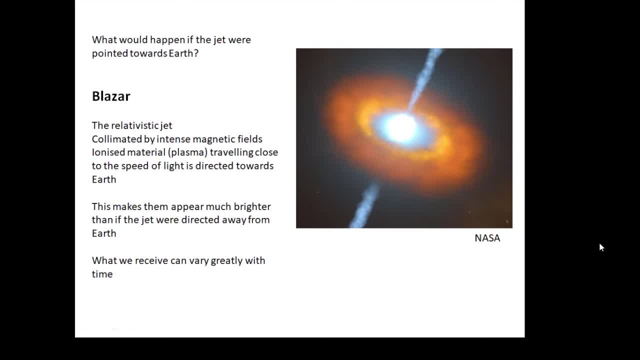 A little bit like a lighthouse. So it's an active galaxy, with the jet is pointing towards the Earth. Okay, It's directed towards the Earth. Imagine a lighthouse And some of them as they rotate. the amount of radiation that we receive can vary greatly with time. And this is a blazar blazing at us.